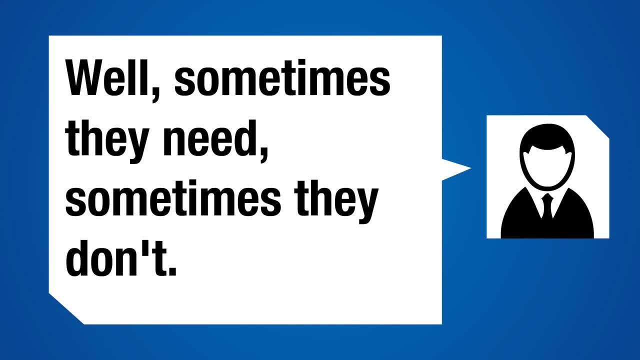 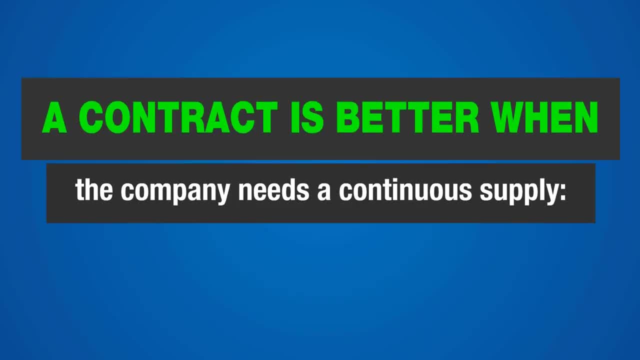 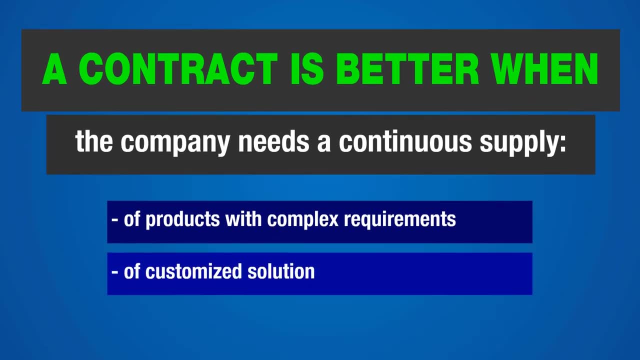 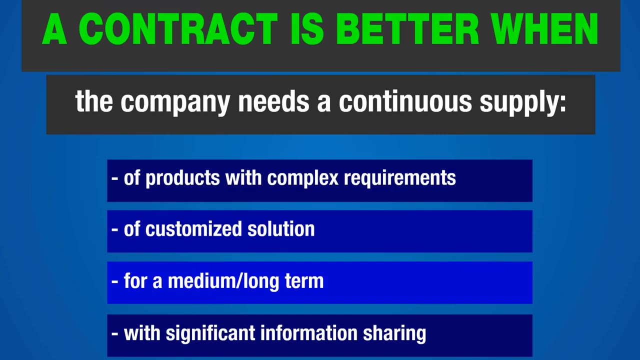 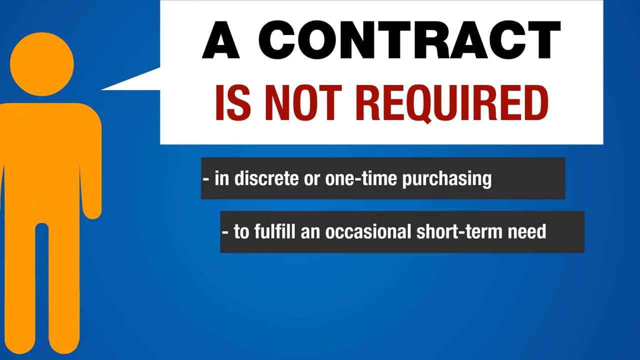 Well, sometimes they need, sometimes they don't. A contract is better when the company needs a continuous supply of products with complex requirements Of customized solutions with significant information sharing for medium to long-term commercial relationships. When a contract is not required and one-time purchasing to fulfill an occasional short-term need in a simple. 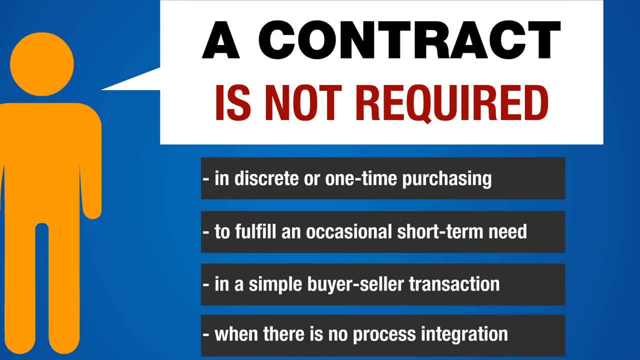 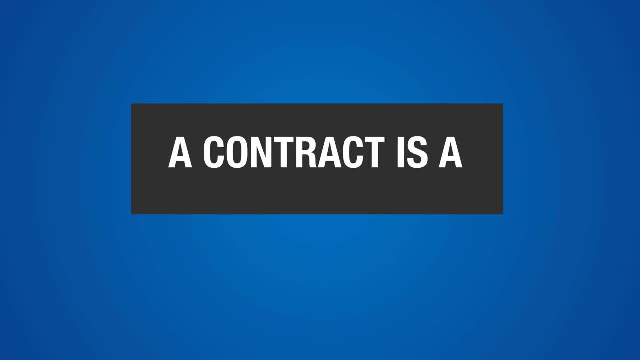 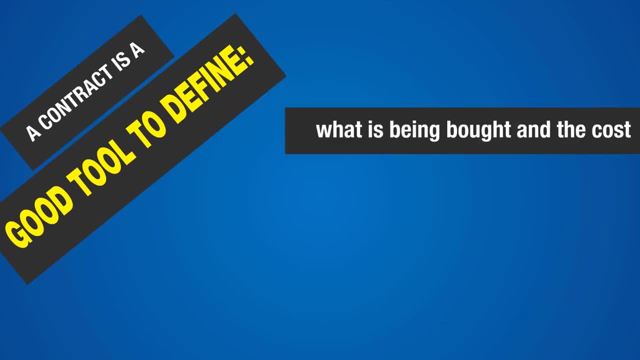 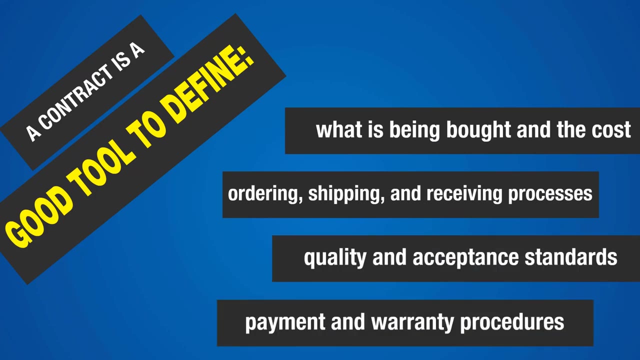 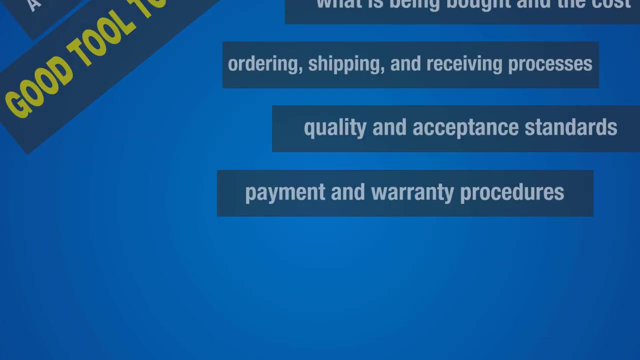 buyer-seller transaction. when there is no process, integration Contract is a good tool to define what is exactly being bought and its cost. The operations process is for ordering, shipping and receiving, to define quality and acceptance criteria, to establish payment and warranty procedures With a. 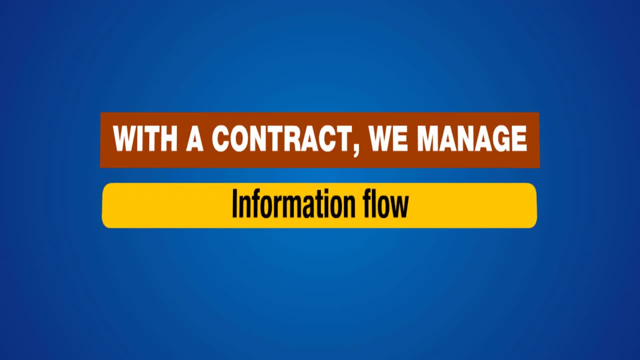 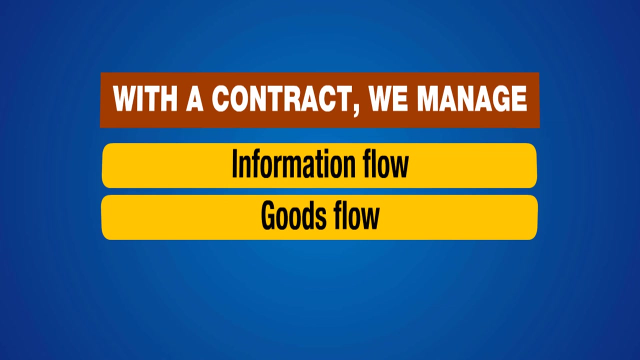 contract companies manage one information flow. The contract establish the communication process: Who sends, who receives, at what time, in what form. also: 1. How communication systems will be integrated, What information will be transferred through the Electronic Data Interface. 2. The goods flow. The contract defines how materials will be ordered, transported, delivered, received and accepted. 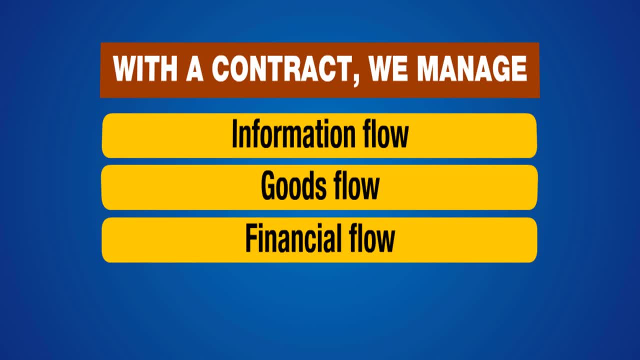 3. Financial flow Contracts describe how and when the payments will be made. 4. Commercial relationship Contracts specify the point of contact, who is responsible for what and the escalation procedure in case of problem. What are the main contract types? 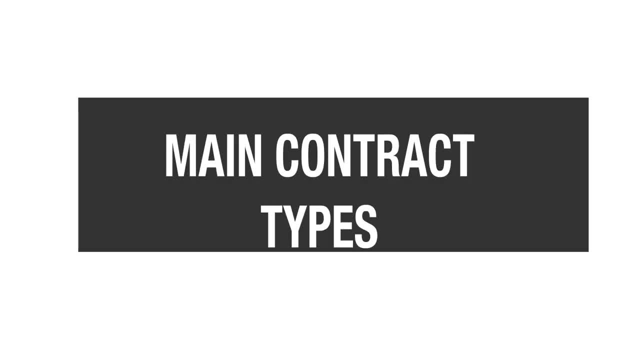 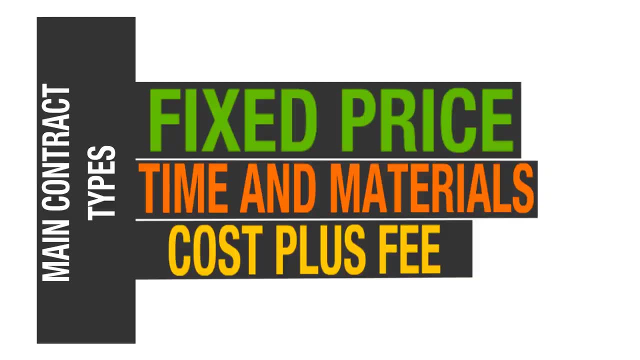 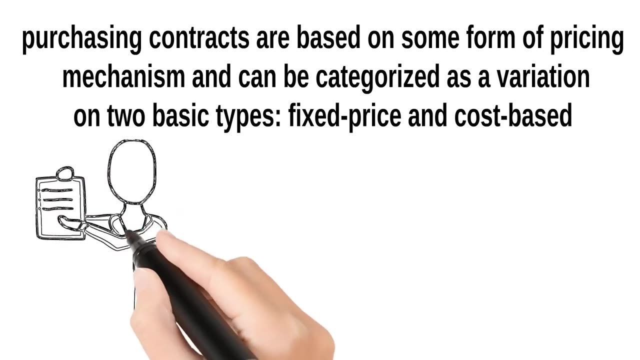 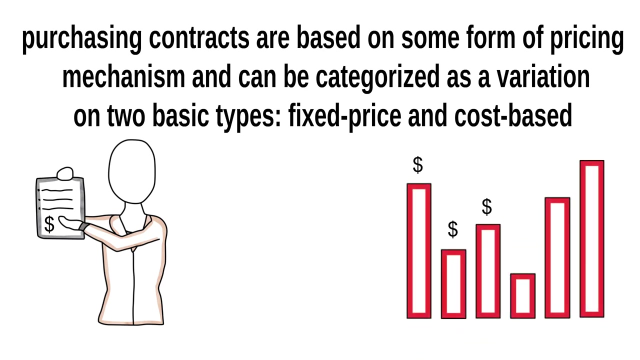 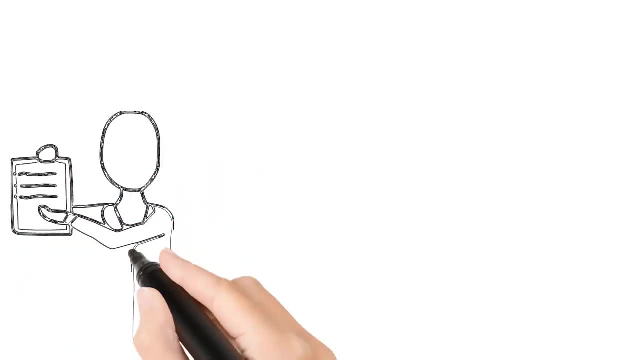 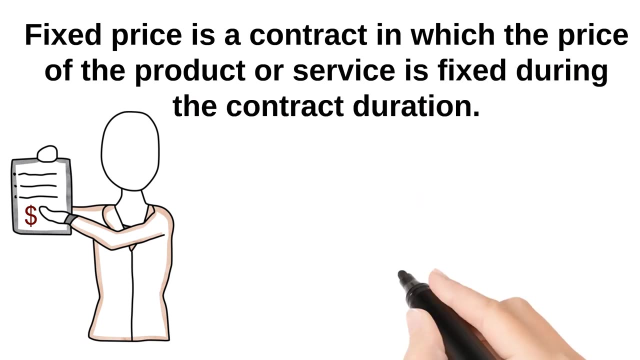 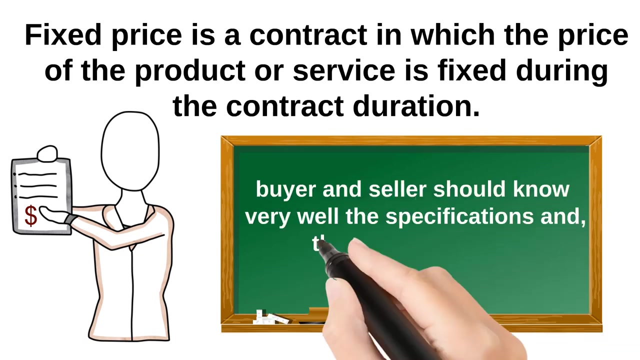 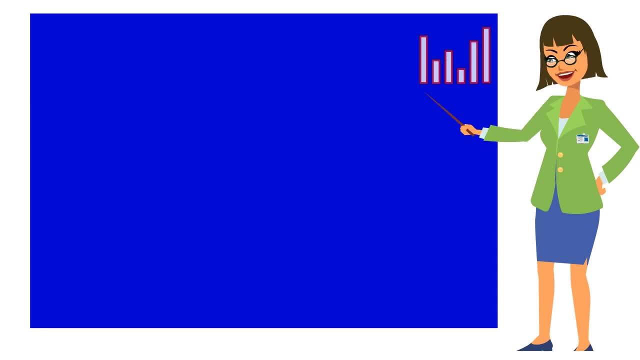 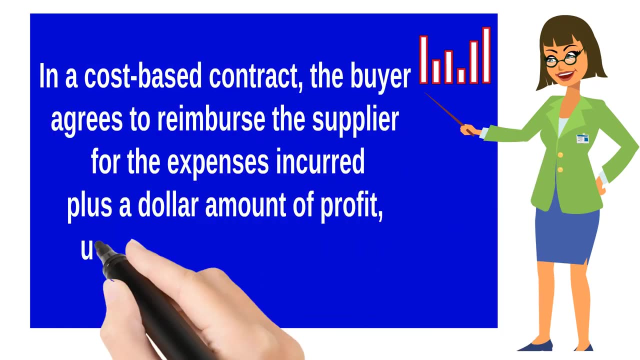 In a cost-based contract, the buyer agrees to reimburse the supplier for the expense in which the product is made, expense incurred during the contract and, of course, plus a dollar amount of profits. To protect against cost overrun, some companies define the maximum cost. the supplier cannot. 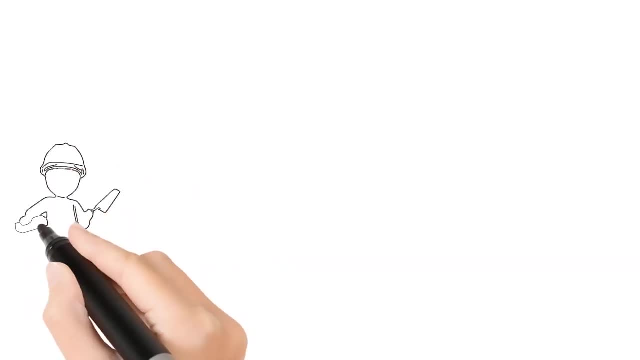 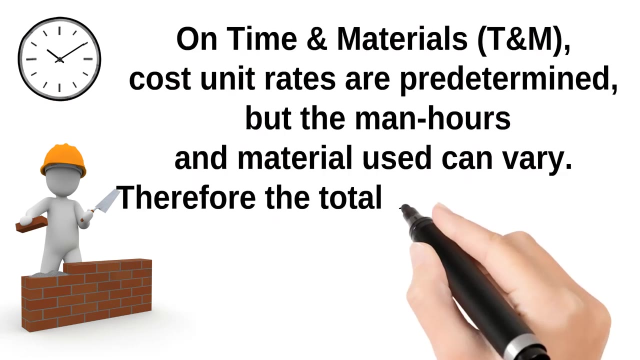 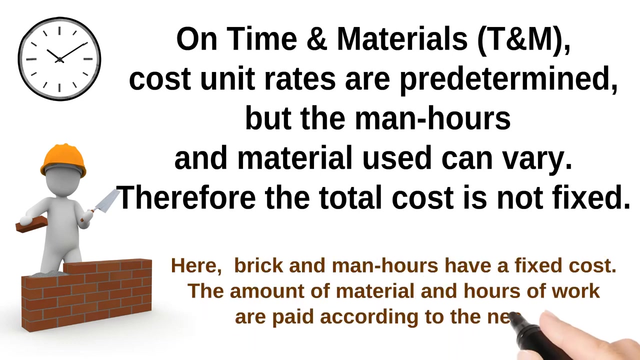 exceed In time and material contracts. the cost unit is predetermined, but labor and material quantity can vary. Therefore the total cost is not fixed, although the unit costs are predetermined. It is a kind of hybrid contract. In this small example, the break, 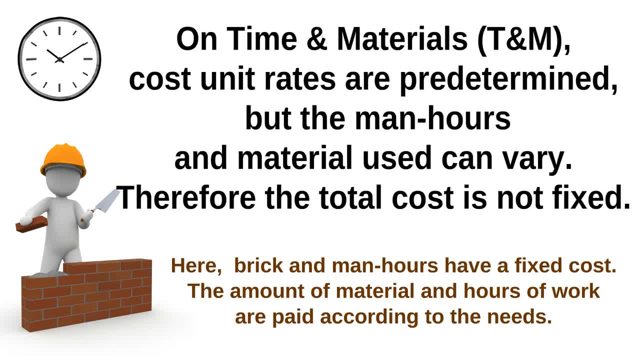 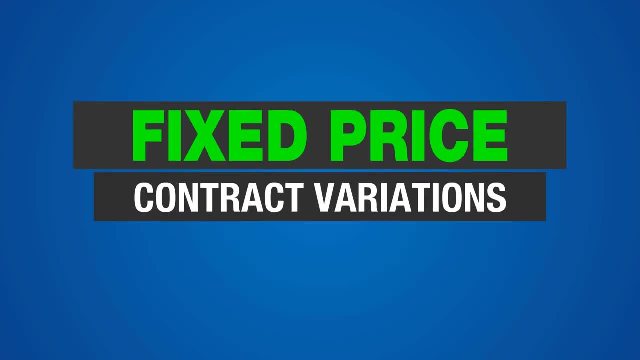 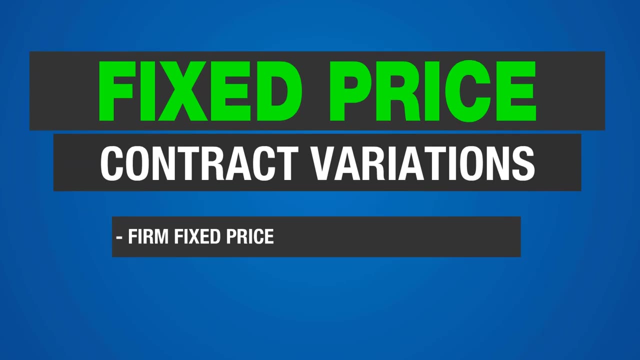 and labor rates have a fixed cost. The total price will depend on the amount of material used and hours worked. Fixed price contracts may have problems to handle change and quality assurance. There are small modifications that can be implemented to reduce the most common risks. 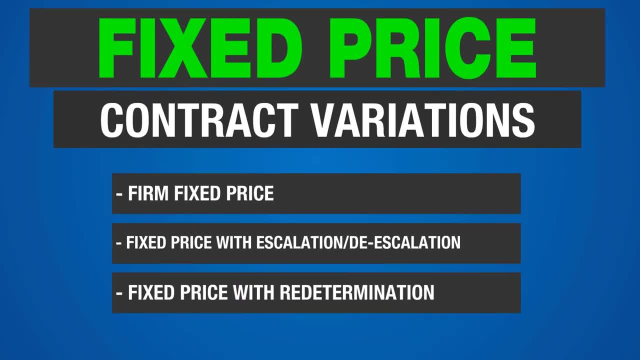 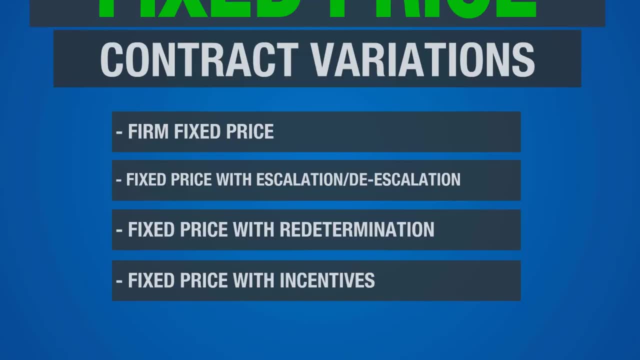 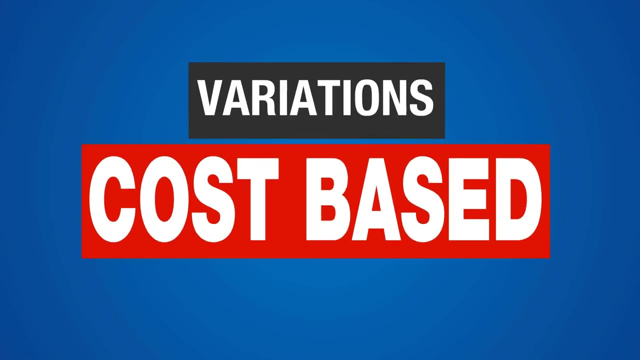 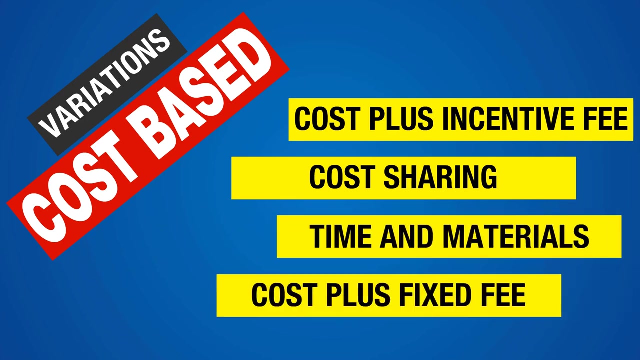 The main varieties are intended to provide formal mechanisms to change prices and to provide incentives for quality. The major challenge in cost-based contracts is the risk of cost overrun. Sometimes it is nice to change some aspects to motivate contractors to keep the costs low. Financial incentives are usually very effective. 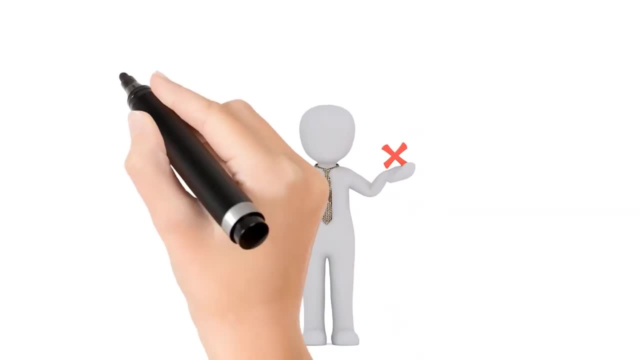 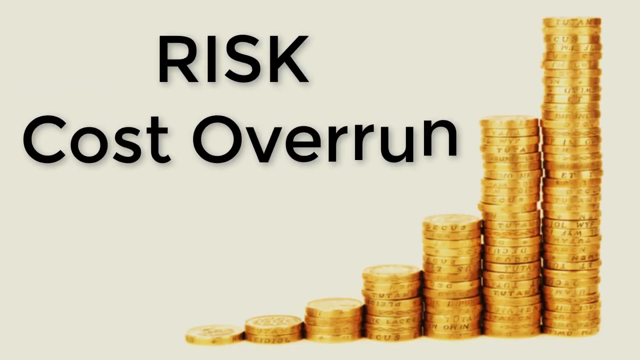 What are the advantages and risks of each contract type? Cost overrun- The risk that the cost exceeds the contract budget, estimated cost or target value is much higher in cost-based contracts. To mitigate the risk, the buyer should put some additional effort in the contract administration, expenses control and maybe include saving incentives for the supplier. 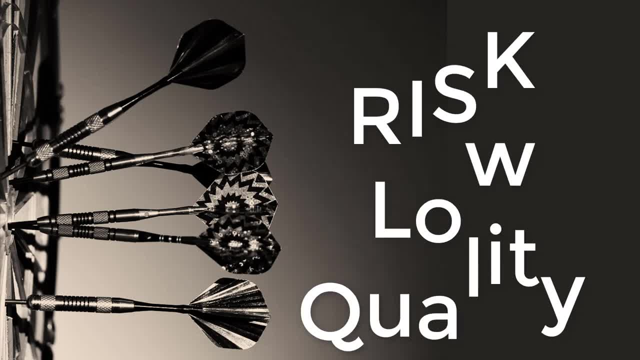 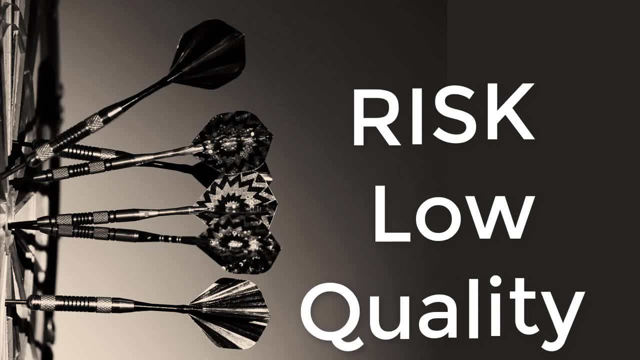 Low quality. In fixed-price contracts, the potential risk of low quality is higher because the price is fixed and the vendor may be forced to reduce costs, What may affect the product or project quality. To mitigate these risks, the buyer should have well-known specifications and include quality standards. 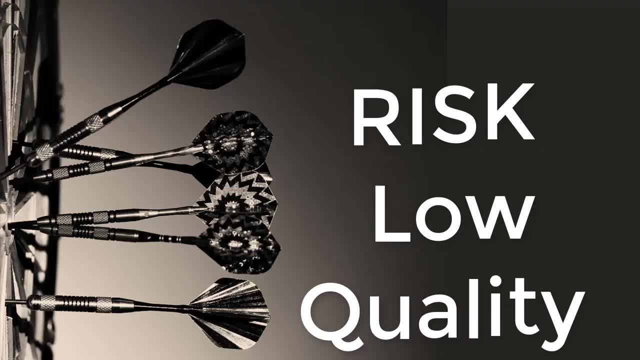 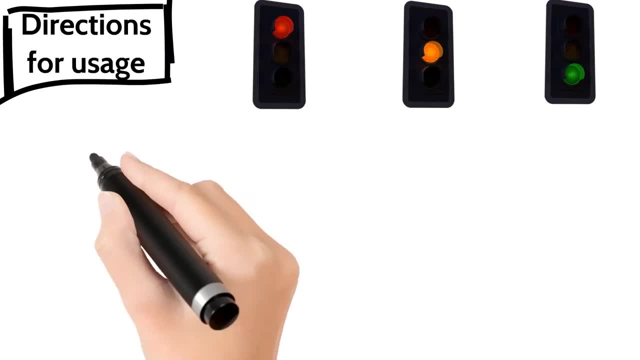 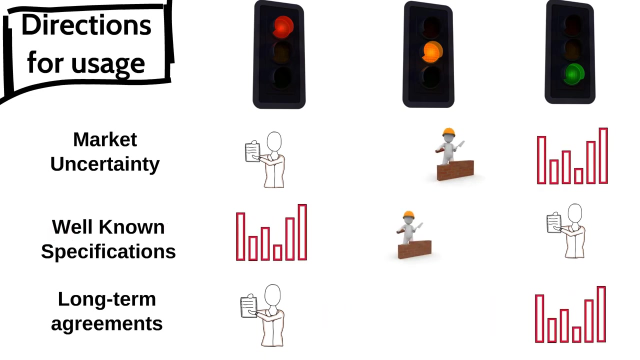 A checked price is considered by the buyer and proportional processing is determined by each force to make the product a good match. What Lobby Theoretical enterprise? Fixed price contracts are not recommended. Long-term contracts also bring changes, naturally. therefore, fixed price contracts should be. 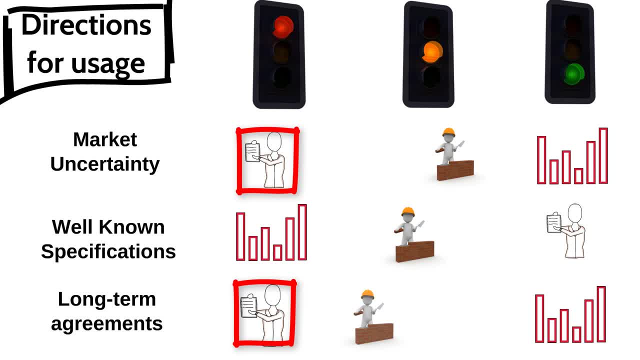 avoided. In case the company has an in-depth knowledge and experience about the product and are able to develop very well-detailed specs, fixed price is a good alternative. On the other hand, cost-based contracts can be more suitable when there are high uncertainty. 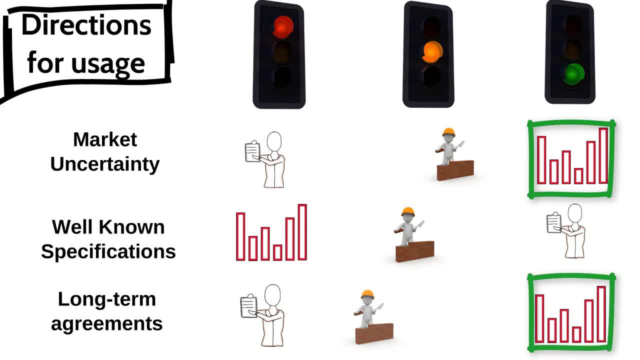 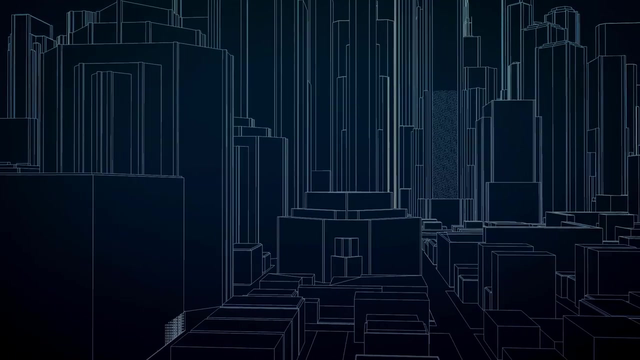 and long durations. The time and materials contracts are an intermediate solution that combines elements of fixed price and cost-based contracts. It has fixed price for work units and materials, but also accommodates changes in the scope and workload. In this video, we presented the main concepts of contract management.